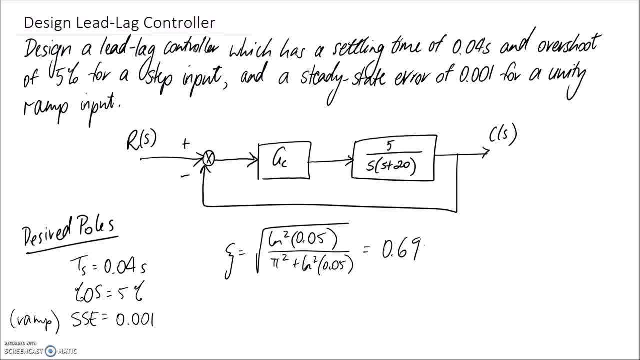 And if you type this into your calculator, you find out that it needs to be 0.69 for the damping ratio. If we then apply our settling time equation- remembering that this is an approximation equation- we should be able to rearrange it for omega n, our natural frequency. 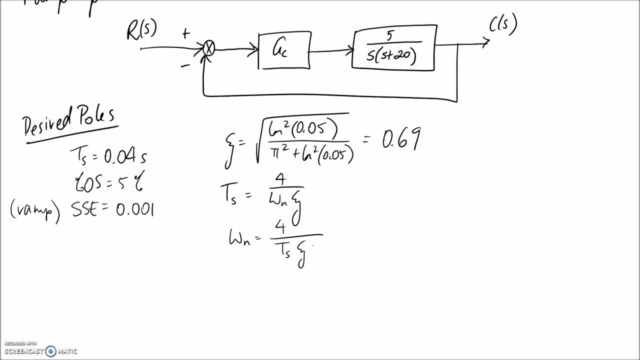 And because we know the settling time that we're aiming for and we've just figured out zeta, we should be able to get an answer for what the natural frequency is, And it comes out to be about 144.9 radians per second. 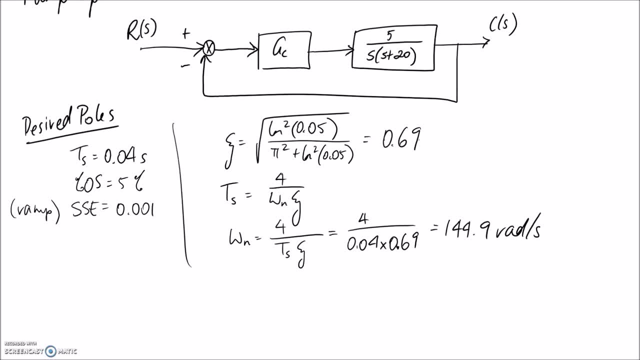 So, based on these two quantities, the damping ratio and the natural frequency, we should be able to figure out these desired poles. So the general form of the equation looks like this for a second order system, And if you substitute in omega n as being 144.9,. 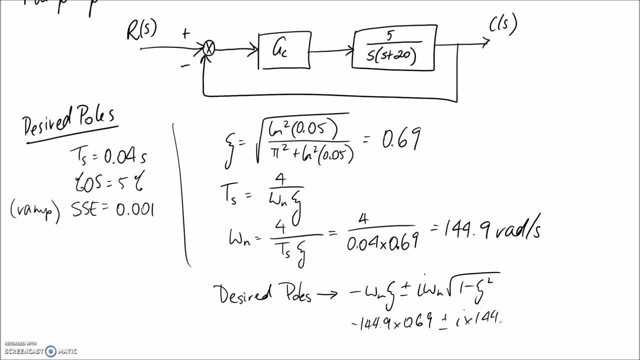 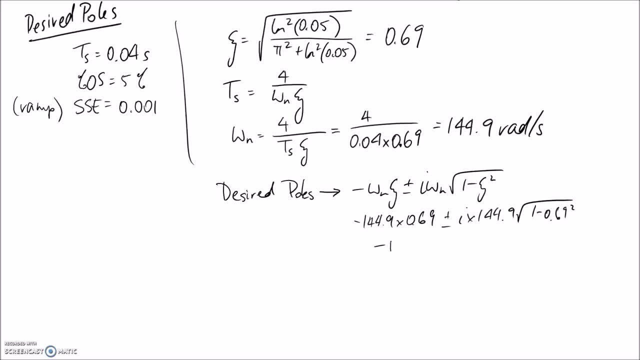 and zeta as being 0.69, you end up with your desired poles being at negative 100 plus or minus about 105i. Alright, so our steady state error criteria isn't going to come into it until toward the end, when we design our lag part of our controller. 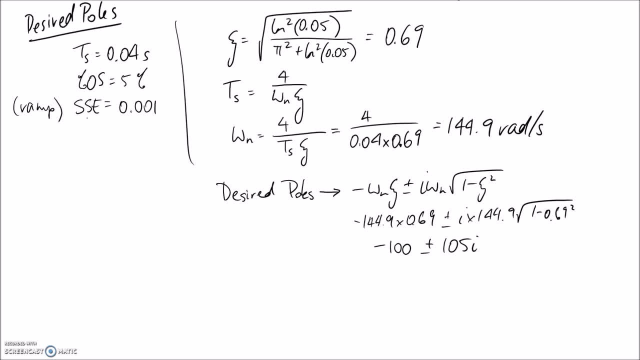 And that's when we focus on making sure we can meet that steady state error requirement. So the next step becomes needing to design our lead controller And for this part of the process, we're focusing on making sure that the root locus of our system. 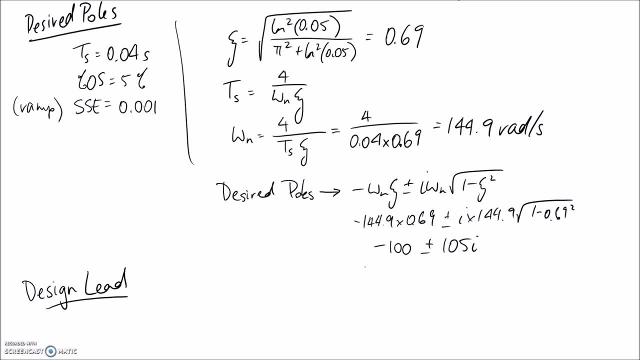 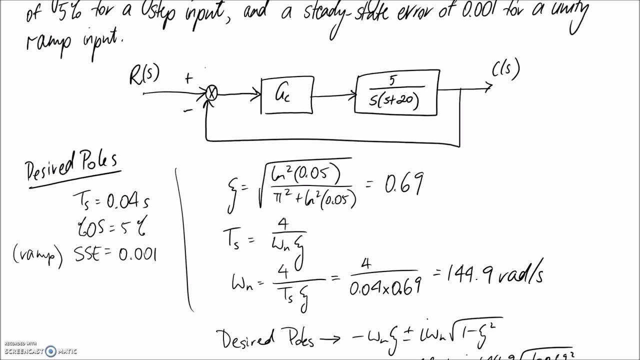 passes through these desired poles, so that we're then able to pick up the value of k. That will ensure that our closed root response is doing what we want it to do. So let's write out our open loop transfer function based on what our system looks like here. 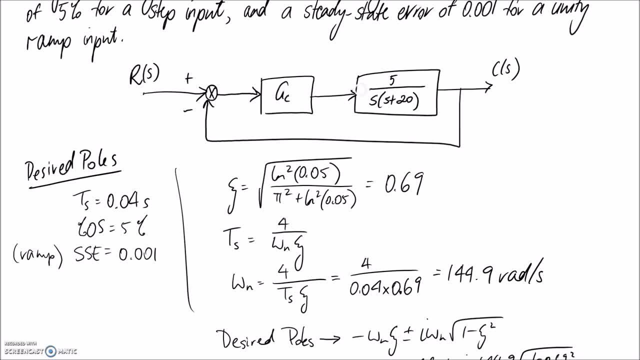 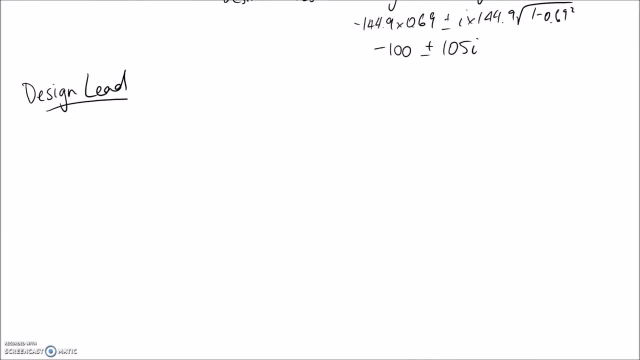 So open loop means that we don't consider the feedback, We're just looking at the top line. So it's going to be gc multiplied by this block here. Alright, so that's our starting point. Now for the lead controller, that's going to mean that gc takes this form here: 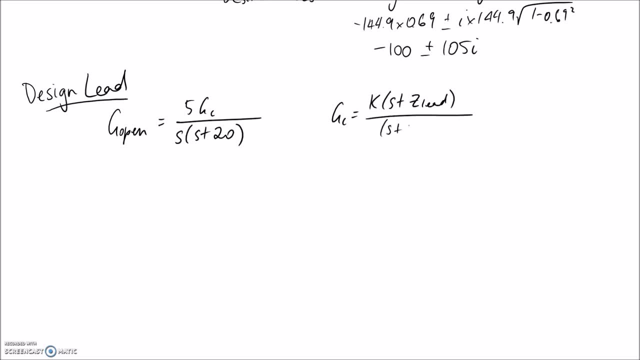 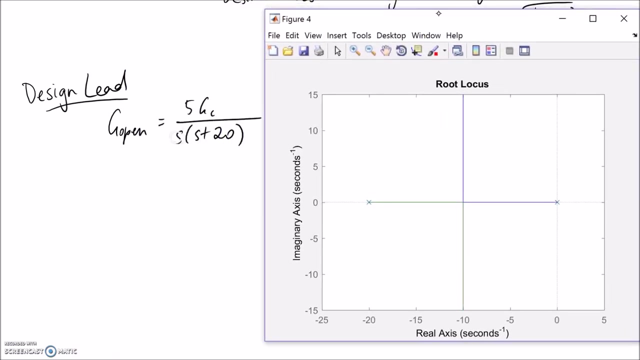 So we need to introduce a 0 and also a pole, such that we end up with these desired poles sitting on our root locus, Because if you look at our root locus as it stands at the moment, we have a pole at 0.. A pole at 0.. 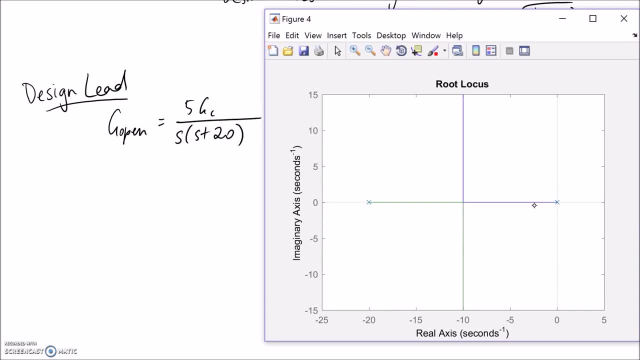 And a pole at negative 20.. And this here is the one I've plotted from MATLAB. That's the pole at 0.. That's the pole at negative 20.. And you can see, these root locus lines go nowhere near our desired poles. 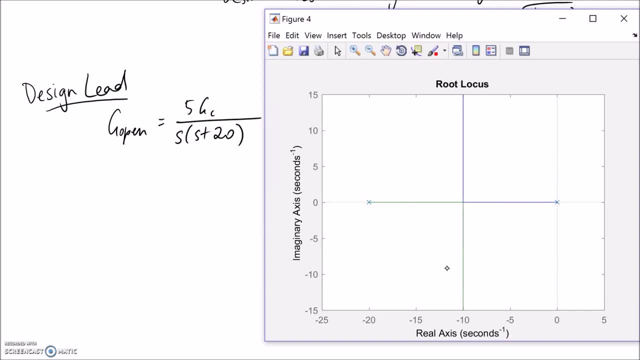 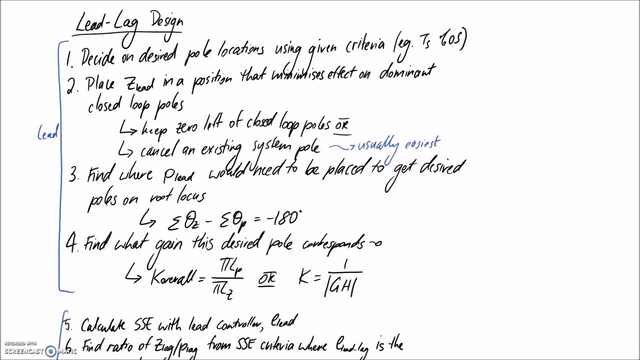 which were at negative 100 plus or minus 105. So they're way out over here somewhere. So this is where we need to place our 0 and our pole such that we get our root locus passing through our desired poles. So this step here, it tells us that we can place a 0. 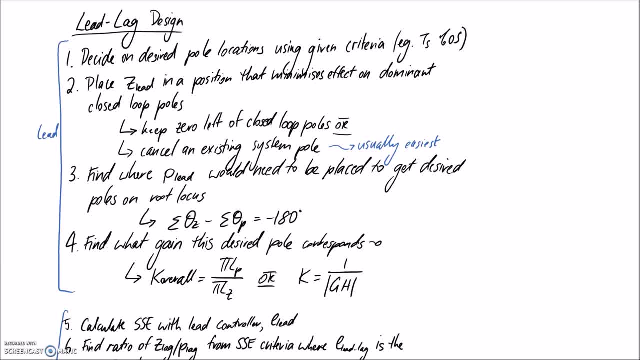 in a position that minimises the effect of our dominant closed-loop poles. So you have two different choices. One of them is to keep the 0 as far to the left as possible of the closed-loop poles because, remember, the further something is from the imaginary axis. 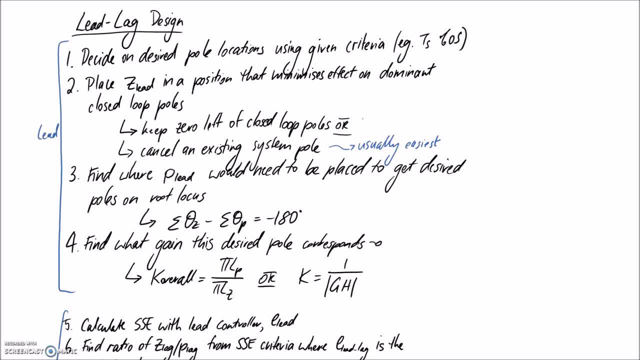 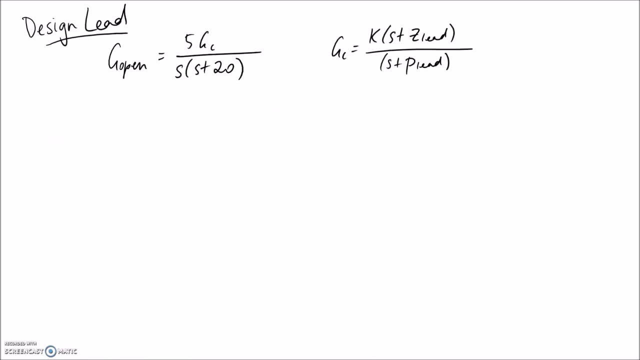 the less impact it's going to have on your response. The other option you have is to cancel an existing system pole, and that means that you end up with pole 0 cancellation, And this is usually the easiest option. So that's the one that I'm going to go with in this example. 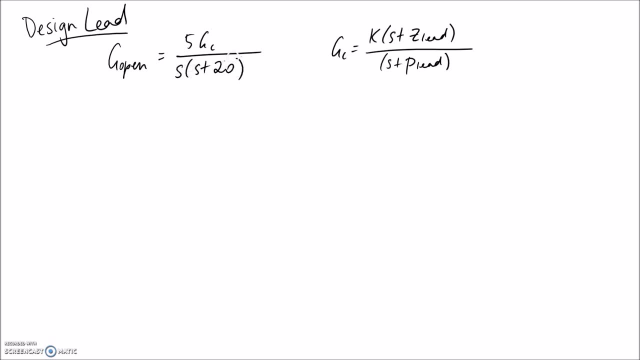 And we can see that we have a pole at 0 and a pole at negative 20.. So I'm going to go with cancelling this system pole. So if we draw out what our root locus diagram is going to look like, Okay, we have the pole at 0.. 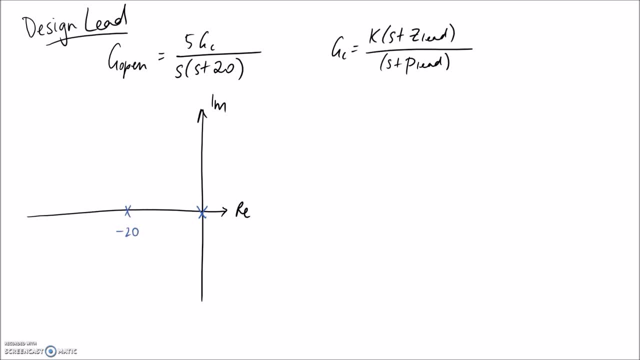 The pole at negative 20.. This is not going to be to scale These two here. the red ones are our desired poles And we know that that's at negative 100 plus or minus 105.. Okay, so these are the desired ones. 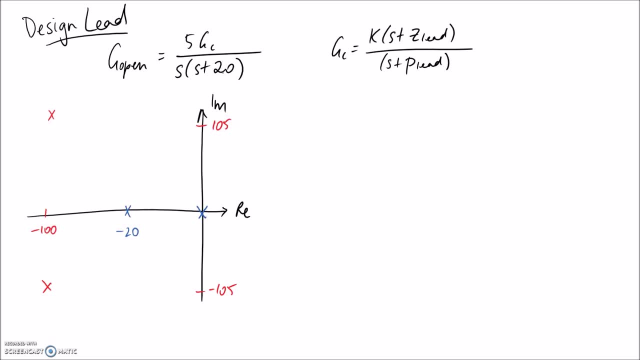 Alright. so if I'm going to cancel out this pole at negative 20, that means that I'm going to end up with a 0 on here. So I've just led my lead. It's going to be 20 in this equation. 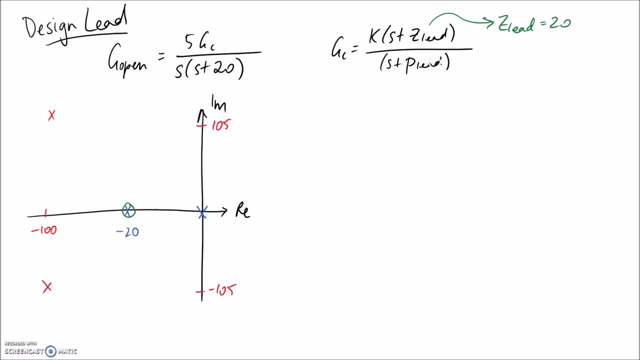 So that's that one. Now, what we need to do is we need to figure out what the corresponding p-lead needs to be. So let me draw it just as a value out here. Put an x for it. Okay, This is that negative p-lead. 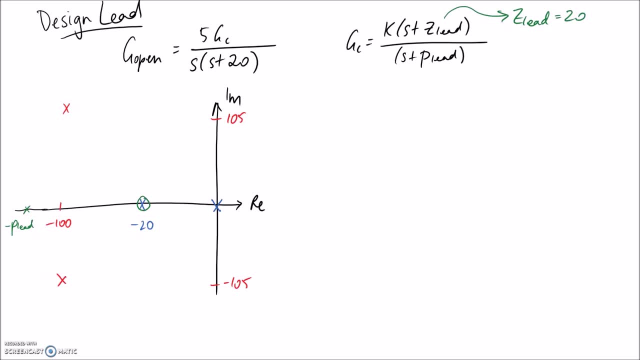 And we need to solve for where that is. So I'm going to use the graphical method to work this out, And that means that we pick one of our desired poles. So I'm going to pick this one here, And we need to look at the angles made. 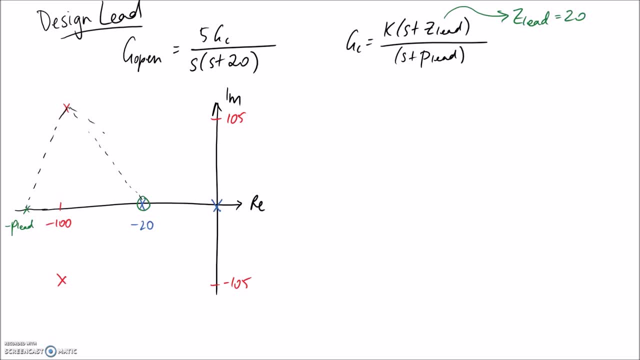 between each of our poles and zeros and that desired pole. You can equally pick the one down here. You should get the same answer. So you need to measure the angles from the positive real axis and anti-clockwise. So that means that this angle in here 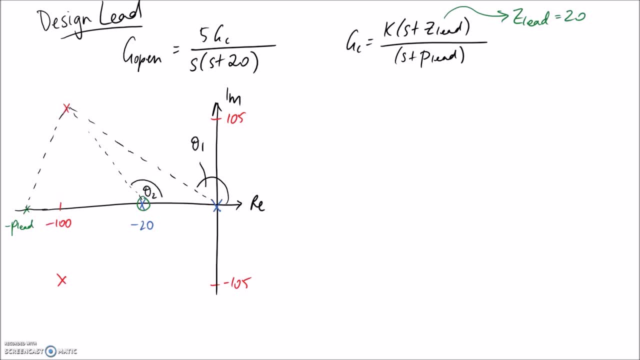 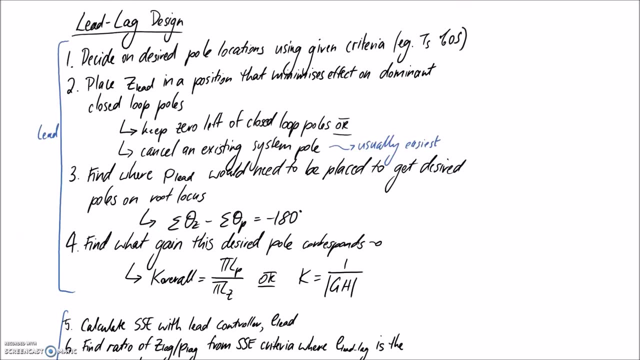 I'm going to call theta 1.. I'll call this one theta 2.. And I'll call this one theta 3.. We can go through and work them out. So this is the equation that we're filling in here: The sum of the zero lengths minus the sum of the pole lengths. 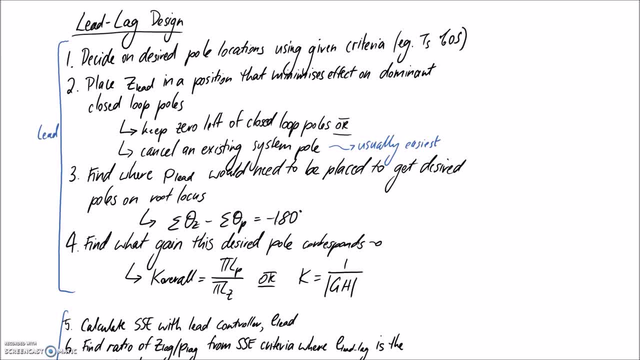 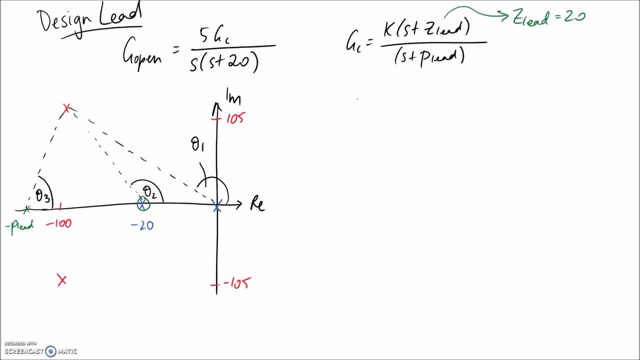 have to be equal to negative 180 in order for our position of interest, which is our desired pole here, to be sitting on the root locus. So let's go through and instead of having these in terms of theta z and theta p, we'll put it in terms of theta 1, 2 and 3.. 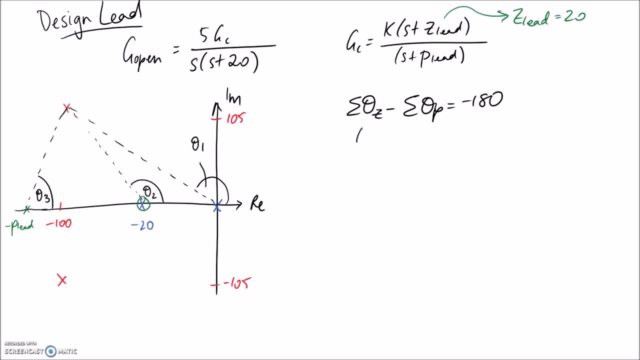 So we only have one zero in our system and that's going to have an angle of theta 2.. We've got three poles in our system at theta 1, theta 2 and theta 3. And what we're going to find is this: 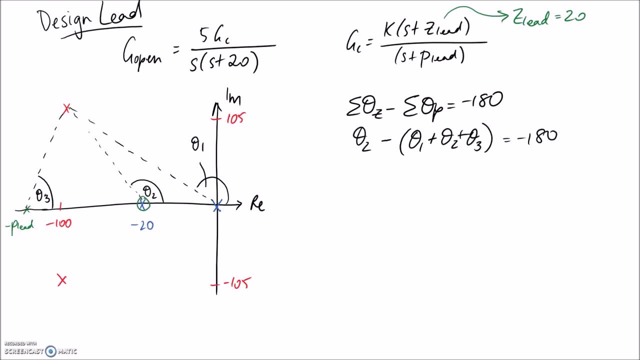 pole: zero cancellation here. It's going to make our lives a little bit easier, because theta 2 minus theta 2 gets cancelled out. In fact, as well the negatives on both sides here are going to cancel out. So we're just left with this. 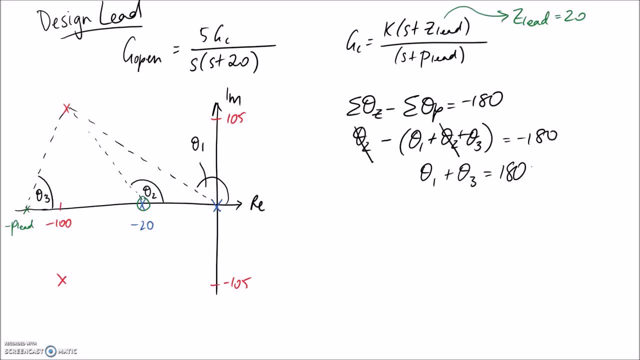 as the equation that we need to satisfy. So let's go through and figure out theta 1 and theta 3.. So I can figure out this angle by taking 180 degrees, which is the number of degrees in a straight line, and minusing away this little piece in here. 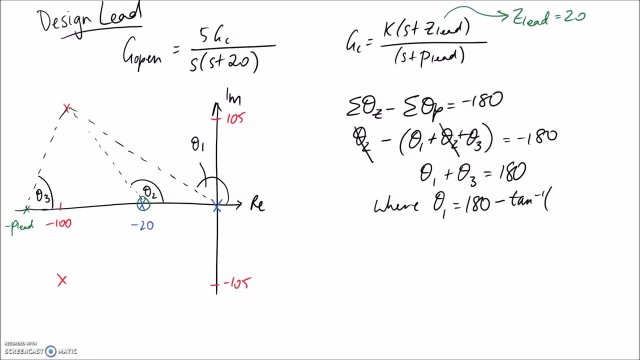 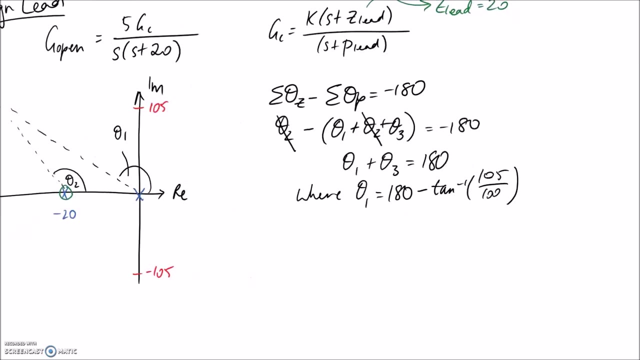 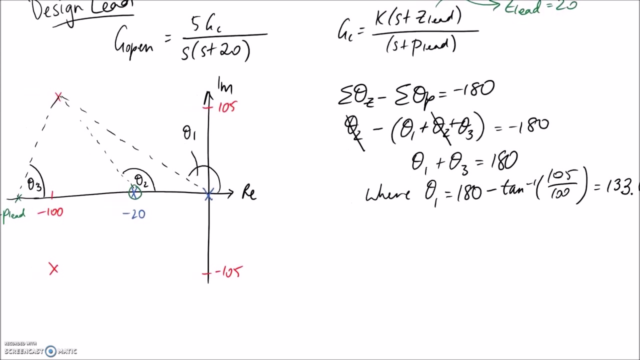 And using my trig, that's going to be inverse tan of the opposite over the adjacent. So the opposite here is 105, the adjacent is 100. And this one works out to 133.63. whoops, sorry degrees, Alright. so now we need to also figure out theta 3.. 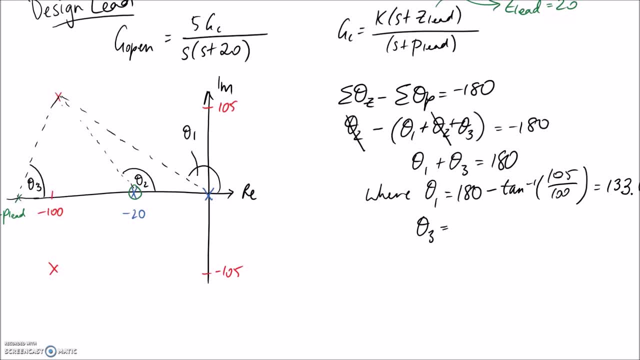 And looking at this angle in here I should be able to just directly apply trig. So it will be tan inverse of the opposite, which is 105 here divided by the adjacent, which is going to be the difference between P, lead and 100.. So there's not much more I can do with that. 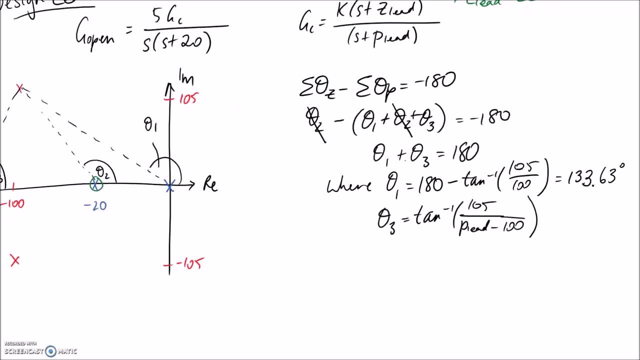 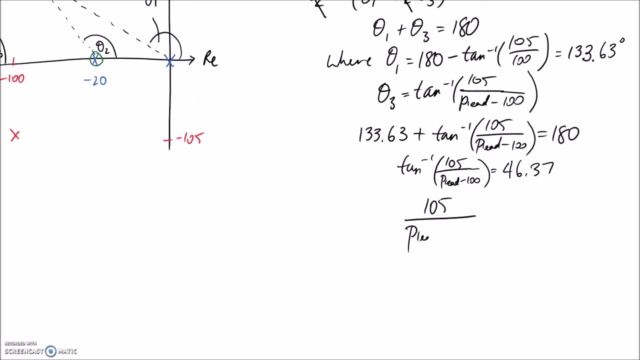 I need to go and sub these back into my equation in order to solve. So taking this away over here, just left with 43.67, is equal to this. If we now take the tan of both sides, we're just going to be left with what's inside the bracket. 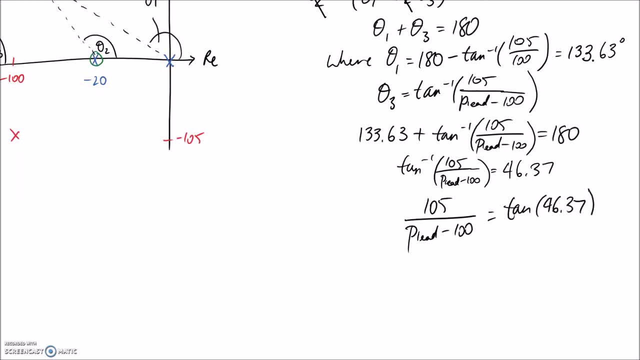 and then this side gets tanned. If we want to get this P lead on its own, I'm going to take it up to the other side and at the same time bring the tan part down. So P lead is going to be whatever this works out to be. 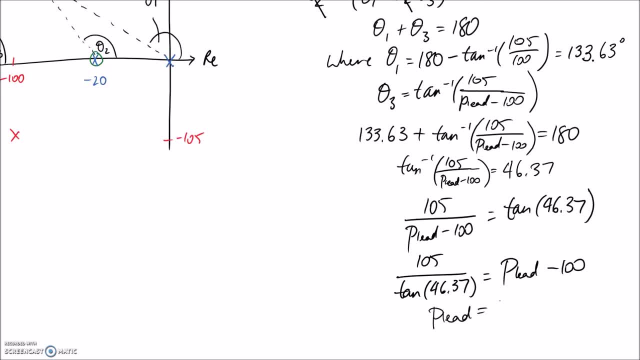 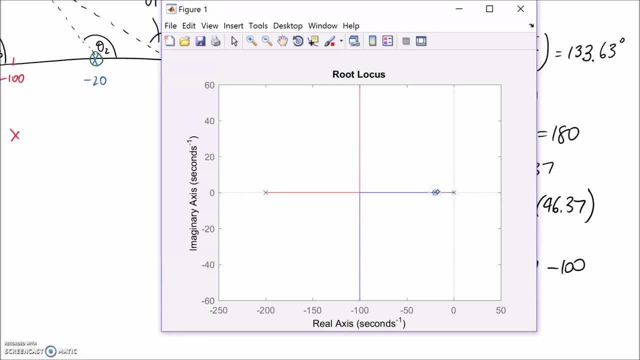 plus 100, and that becomes 200.. Alright, so if you now went and inspected what your root locus diagram looked like, this would be it, So we can see that we still have the original system poles at 0 and negative 20.. We've then got the 0 that we introduced. 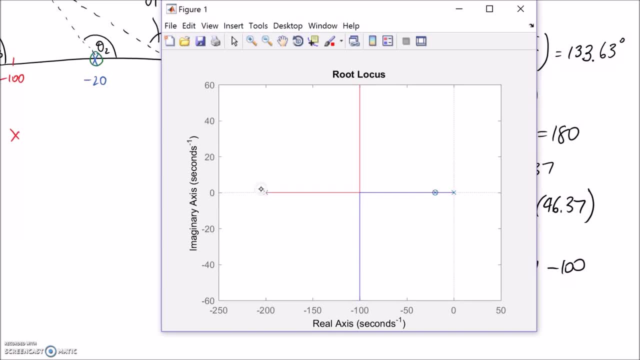 in order to get the pole 0 cancellation effect And then this pole over here that we just calculated to be at negative 200.. So you can see now that these vertical lines for our root locus go through negative 100.. So that would suggest that the point negative 100. 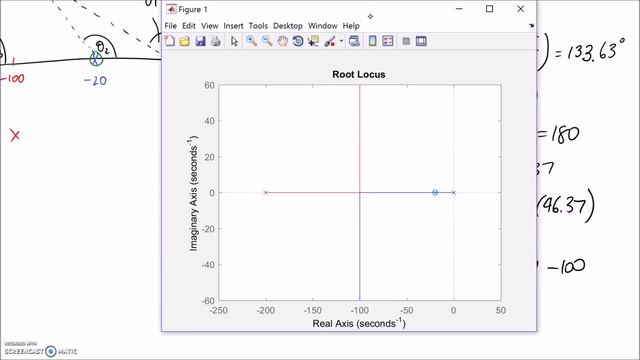 and then plus or minus 105, which would be actually above these, the axis that's shown here. it would lie on the root locus. So that's a good sign. So now we just need to go through and figure out what value of k that corresponds to. 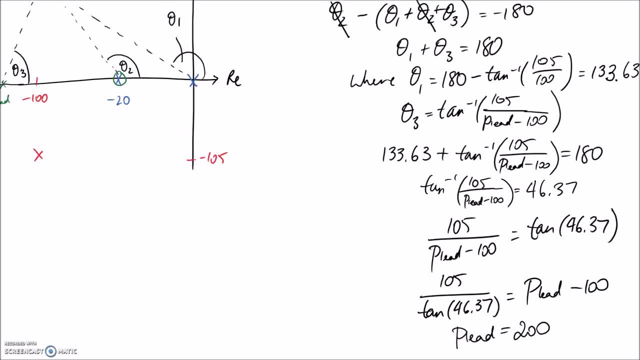 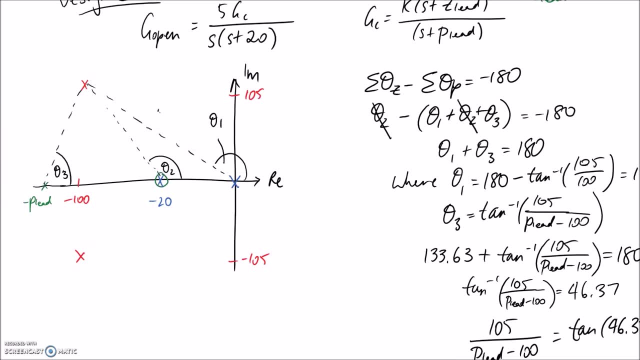 So again, I'm going to go through and use the graphical method for this. So now we need to look at the pole length and the zero length. So let's call the length of this line here L1, this line is L2 and this one is L3.. 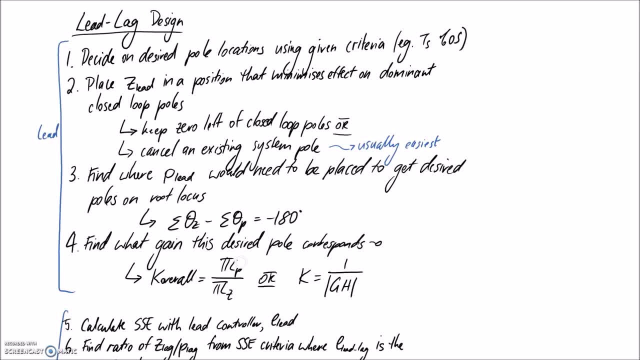 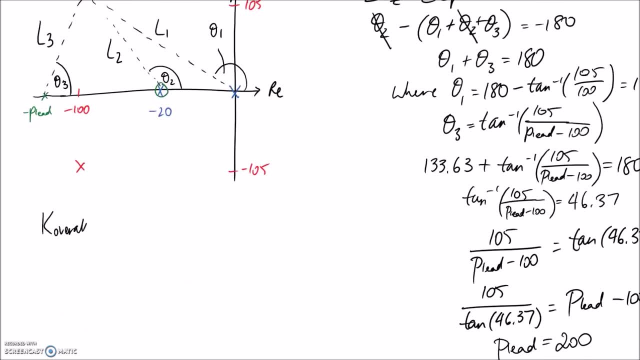 And the equation that we need to apply if we're using the graphical method is this one here: Alright, so Lp is the pole length, Lz is the zero length, and this pi isn't actually a pi. it's supposed to be the product symbol, which means we multiply everything together. 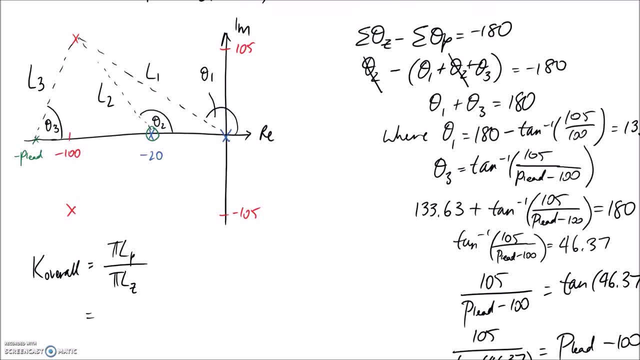 Just like this is the sum of symbol, so we add everything together. So we have three poles and they have lengths- L1, L2 and L3- that we can pop in, And we only have one zero which has a length of L2.. 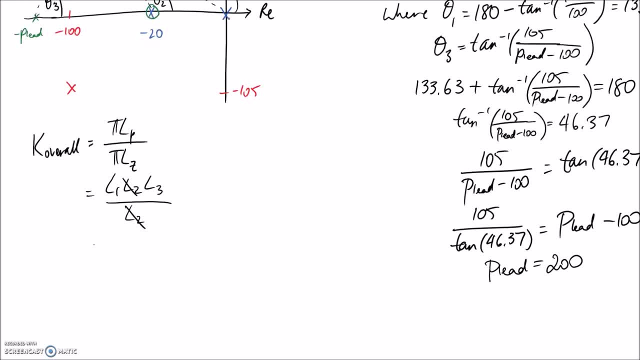 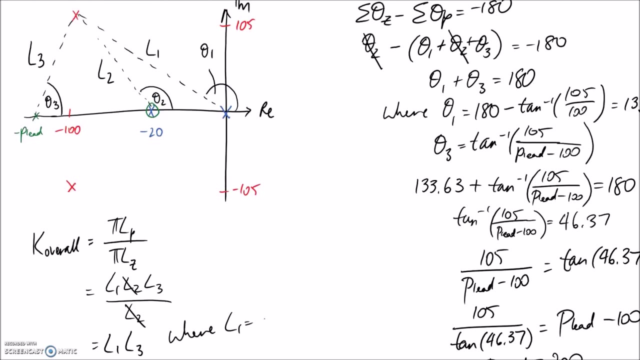 So again we can see the pole zero cancellation happening and we're just left with L1 times L3 and we can go through and figure out what both of these are. Alright, so let's start with L1.. So the length of this line we should be able to get from Pythagoras' theorem. 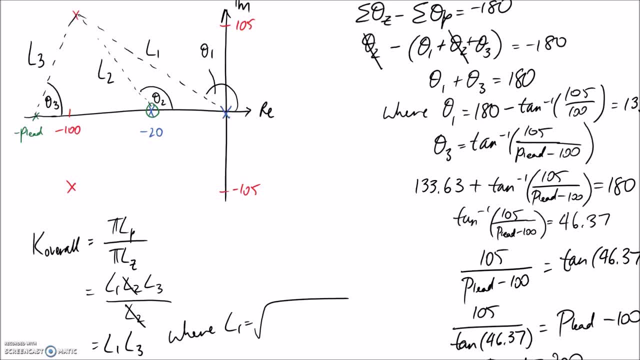 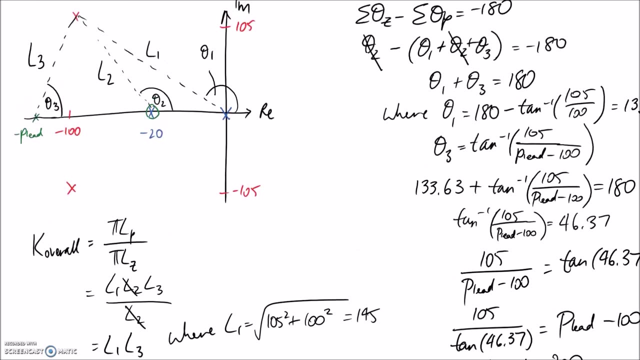 It's going to be the square root of this length, which is 105 squared, plus this length in here which is 100 squared. If you type that into a calculator, it comes out to about 145.. So now, if we go through and do it for L2. 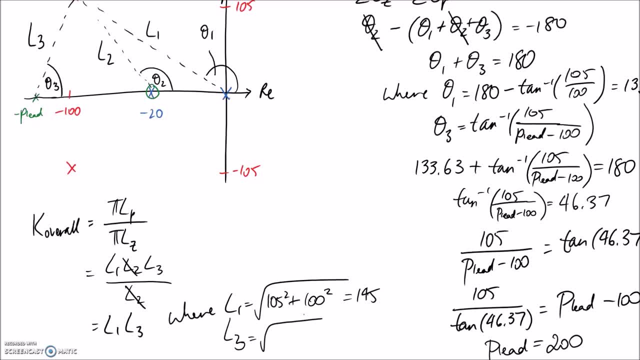 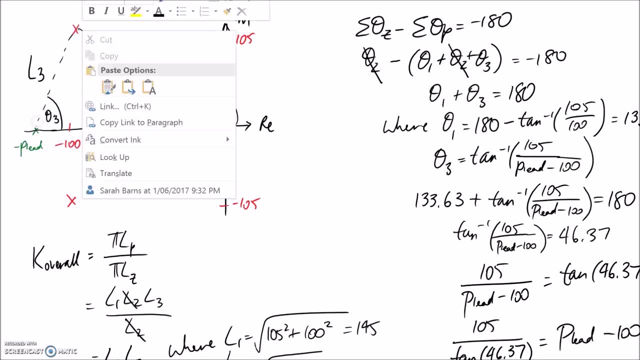 running out of space. sorry, L3, that's the other one we need to fill in this equation. Alright, so L3 is this one here. We now know that P lead is at negative 200.. So the length of here is 105. the length in here is 200 minus 100. 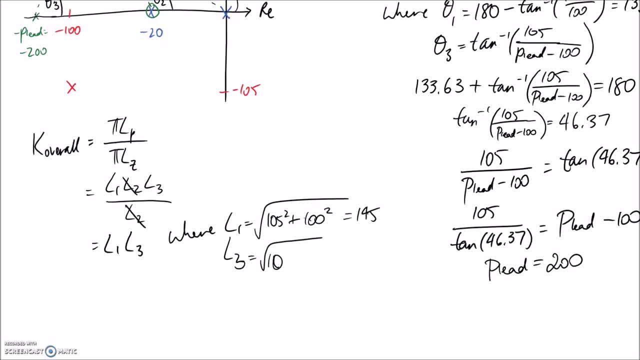 which is 100.. So it's going to be 105 squared plus 100 squared, so it's the same number, 145.. So if we go back and put it in here, it's 145 times 145 and this is equal to. about this: 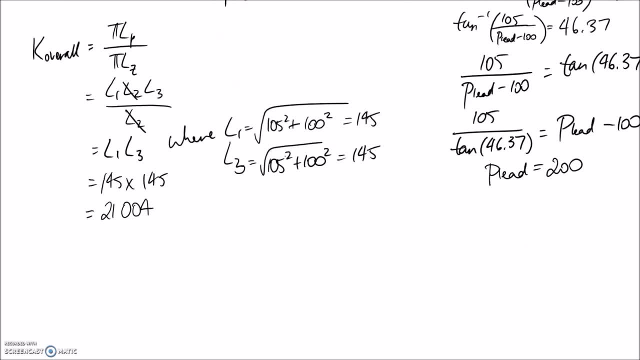 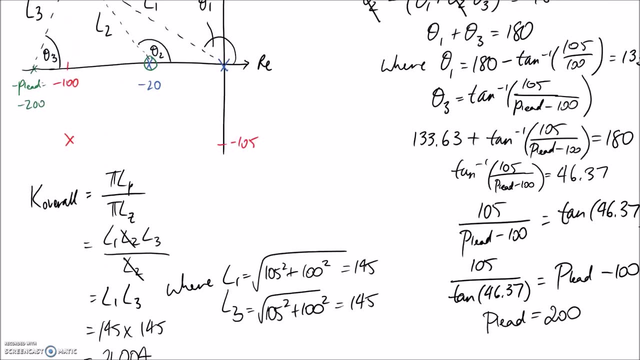 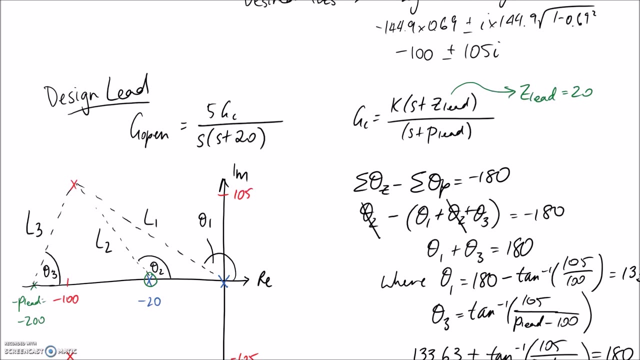 I've carried through a few more significant figures on these numbers. So we said that this number here was equal to the overall gain in the equation. So if we go back up, we're looking for the constant that's multiplied by the whole transfer function on the top line. 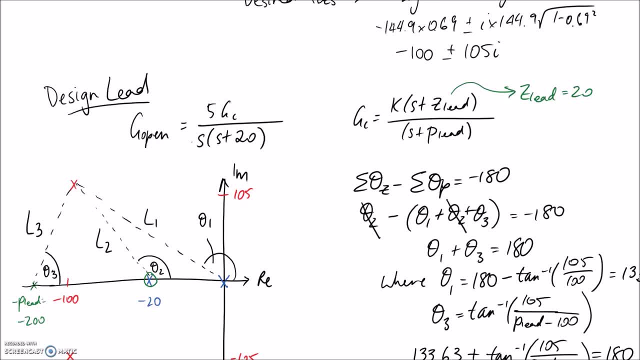 So we can see that in our current form, this is our open transfer function and at the moment, this is our controller transfer function. So we just need to substitute this in for GC and we'll be able to identify the overall gain that we have inside our transfer function. 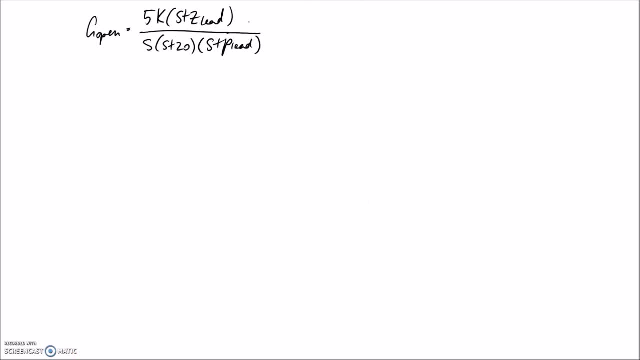 or system, I guess. Alright, so I've copied it down and subbed it in. so now we just need to put in Z lead and P lead, as we have identified them. So we just said that our zero was going to be at 20 and we calculated that our 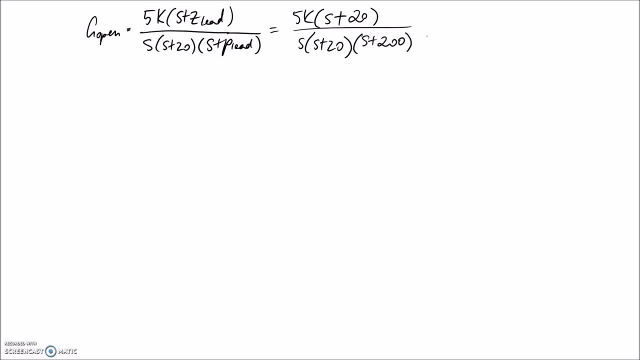 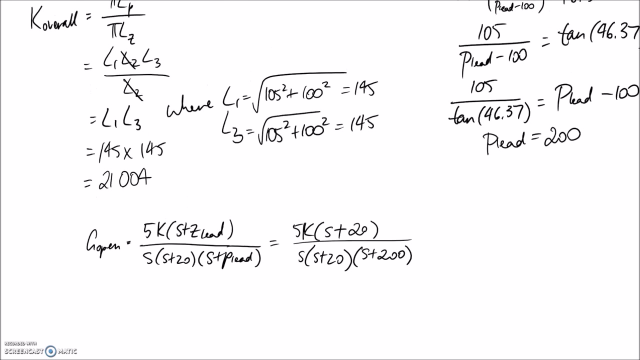 lead pole needed to be at 200 a moment ago. So looking at this equation, we can see that the overall gain in the system is going to be equal to 5 times K, which was the gain within the controller part. So if we jump back up, 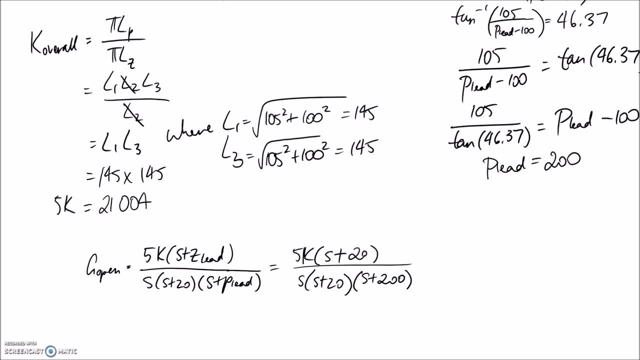 alright, K overall here needs to be equal to 5K. so if we isolate just the part associated with the controller, it's going to be 21,004 divided by 5, and this is 4,201.. So this needs to be the value of K for our controller. 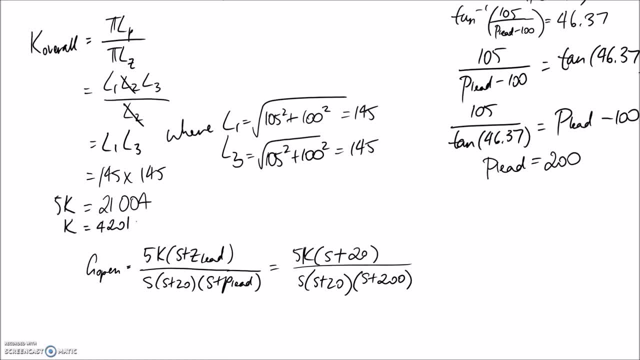 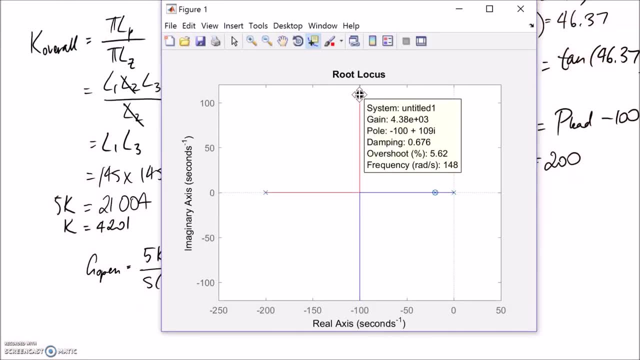 if we're going to get our poles sitting on the root locus. So if I now go back and revisit the root locus diagram that I had in MATLAB, here I'm looking at trying to find my pole, remembering that was at about negative 100 plus or minus 105i. 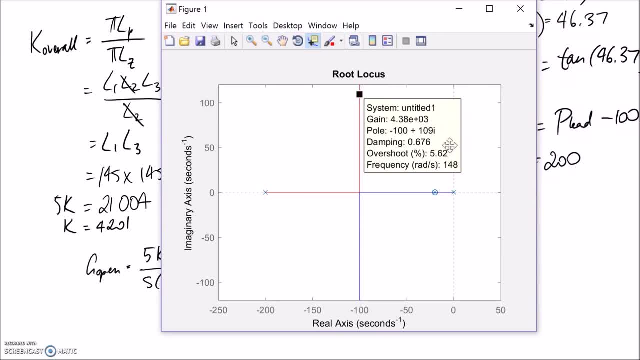 and this is about the closest point I can get to it on the current root locus diagram, since it's a little bit rough in terms of the sketching, But what we can see is that the gain here it's on the range of about 4,300. 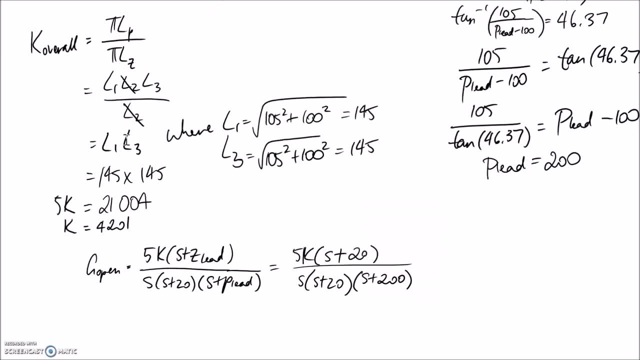 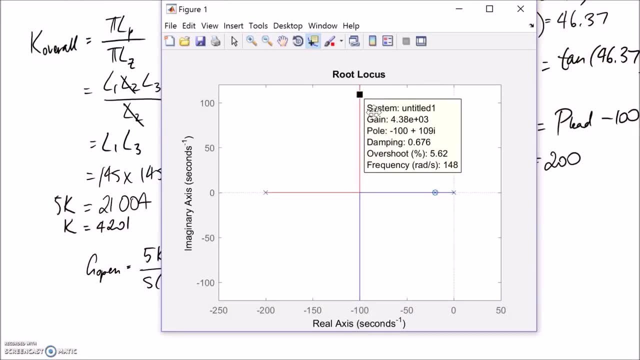 something like that, and we saw that we calculated that our gain was about 4,200. so since it's not quite on the point that we're interested in, but pretty close, I would suggest that MATLAB is agreeing with our manual calculations. So now what we've got is our closed loop pole. 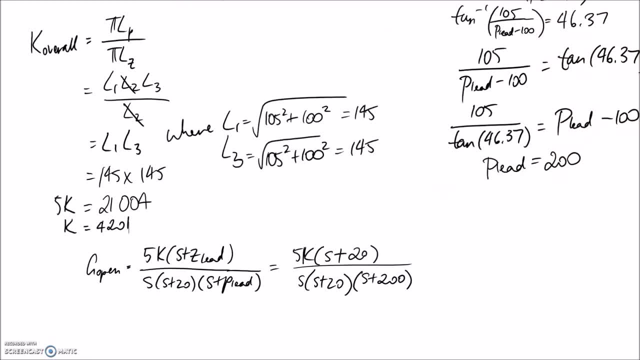 being able to sit on this point as long as we set K to be equal to 4,200 and we keep our Z lead at 20 and our P lead at 200. And our transient requirements, which was the settling time and the overshoot. 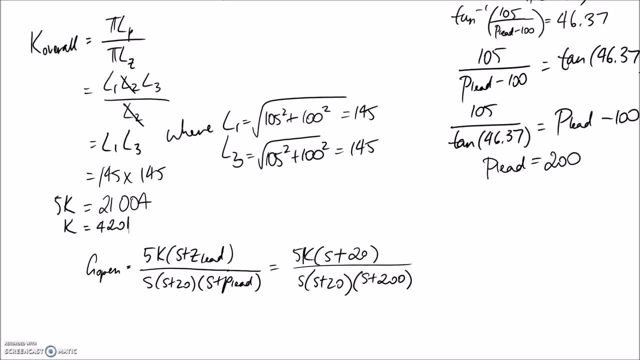 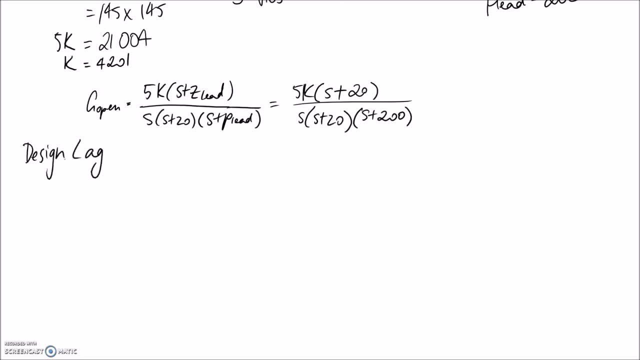 So the next step now is to try and meet the steady state error requirement, and this is where we need to come along and design the lag portion of our controller. So now GC, our controller transfer function. it's going to be what we had before: it's a lead lag. 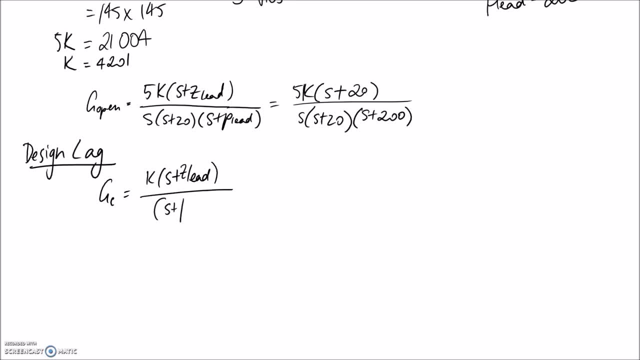 so it needs to be Z lead on P lead. but we're adding in the lag component, so that means that we have our lag 0 and also a lag pole. Okay, and these are the ones that get designed. So at the moment we're at the point where we know K. 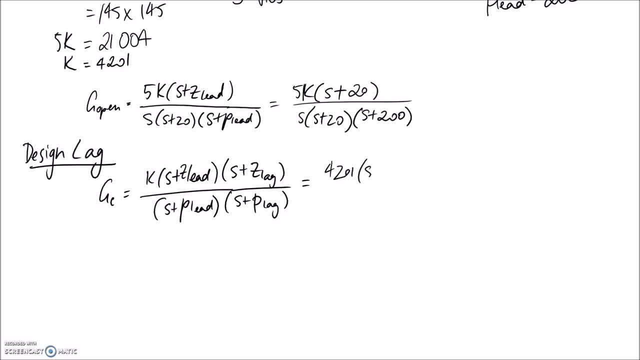 that was the 4,201. we know the lead pole- sorry, lead 0. don't know the lag 0, yet we know the lead pole to be 200 and we don't know what this lag pole is yet. So if we jump back to our 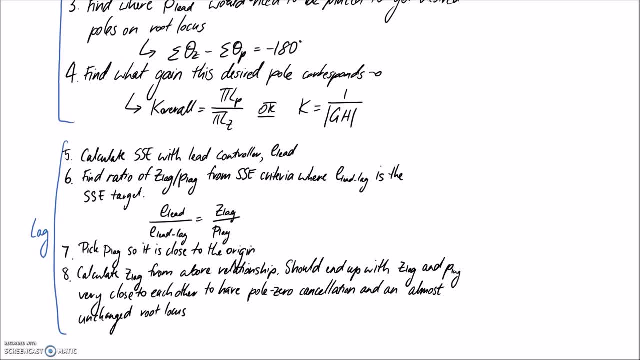 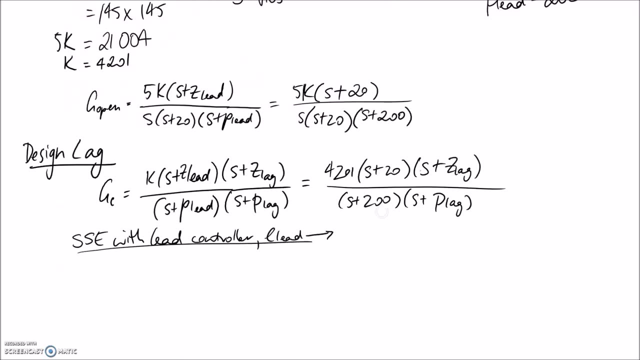 process. the next thing that we need to do is calculate the steady state error that we want to achieve with the sorry that we will achieve with just the lead portion of our controller, Alright. so what that means is we need to go back now and look at the transfer function we had. 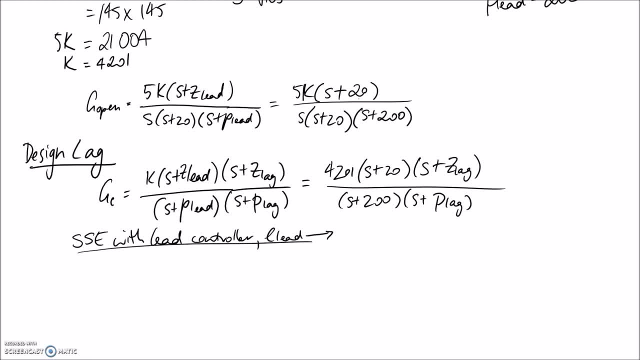 before we put in the lag components. So, looking up here, this is what we've simplified it to at this stage. but what we can see is that, since we have the pole 0 cancellation, those two sections are going to go away and we can substitute in. 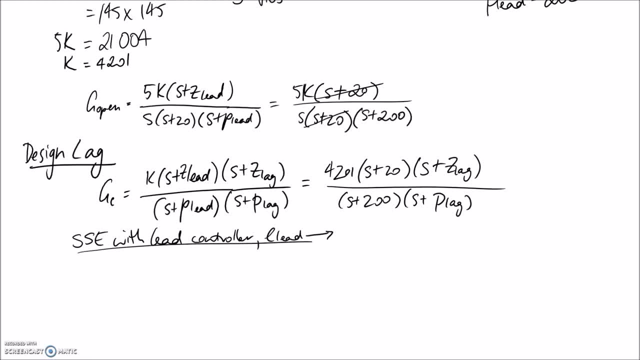 K is equal to 4,200-ish. So if we do that, our open transfer function with just the lead component simplifies to sorry. just this here. Now, looking at this, we should be able to figure out the system type and then we can use our. 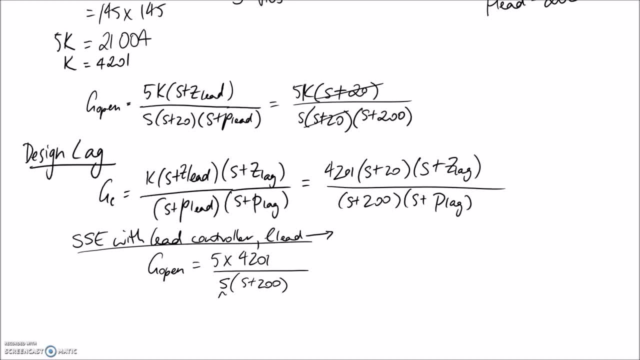 steady state error constants in order to figure out the steady state error. So we can see that we have one S on the bottom line of our equation. That S on its own is like the integrator and since we have one of them, that means it's a type 1 system. 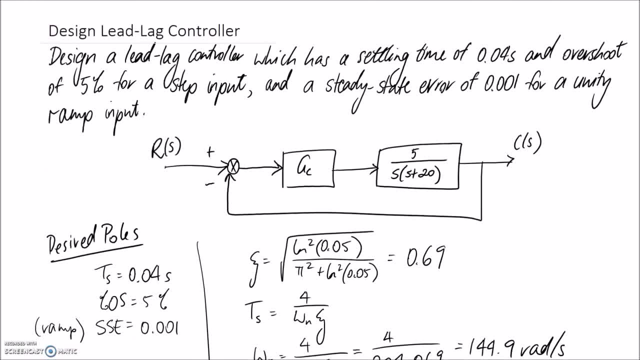 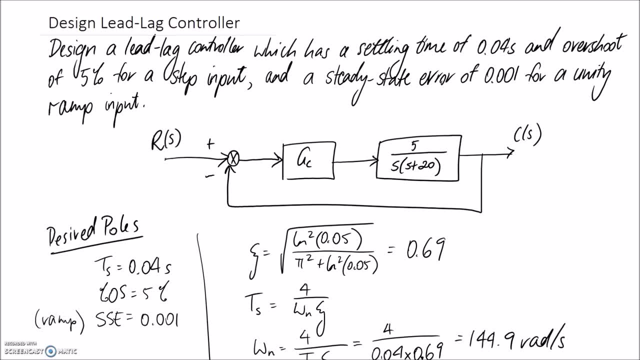 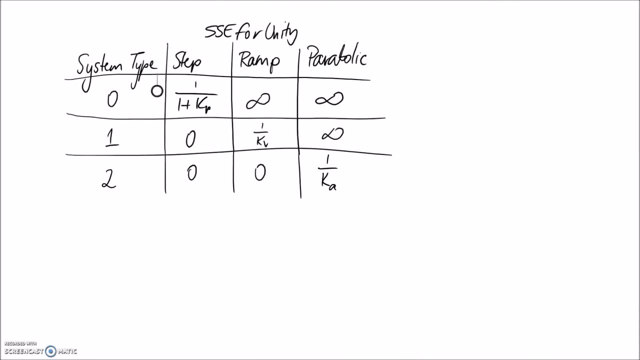 So, remembering that what we're aiming for is a steady state error of this, so a finite value for a ramp input, and in fact it told us it was a unity ramp input. If we scroll down, I've given us the table for working out our steady state errors. 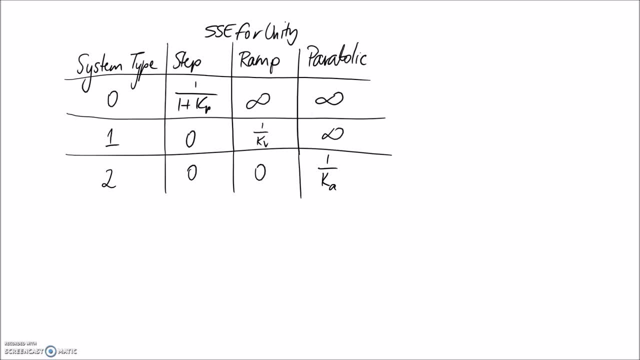 So we just said we have a type 1 system, so that corresponds to this row and we're interested in what's happening for a ramp. So we can see that the intersection is this one here. You can see that this is going to give you a finite value. 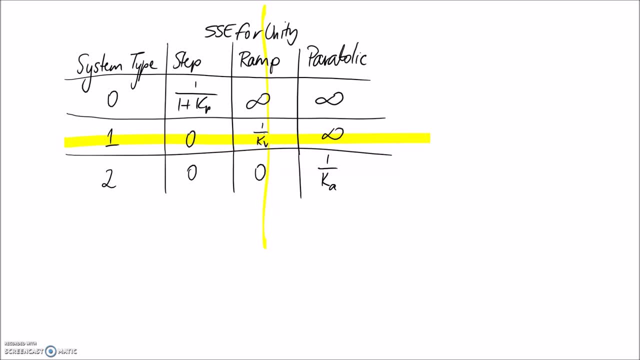 so that means that definitely, the steady state error requirement that we have is achievable. You just need to go through and figure out what it needs to be. So in order to use this, we need to figure out our error, constant kv, and the equation for this is the limit. 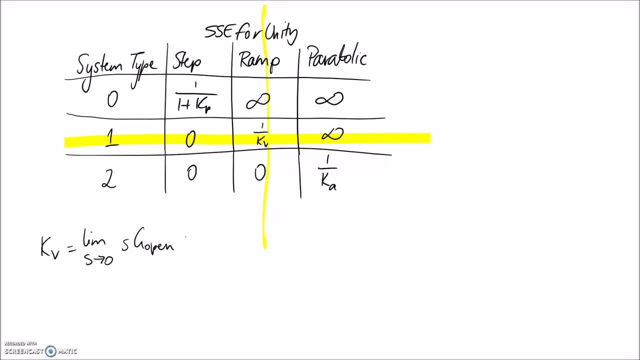 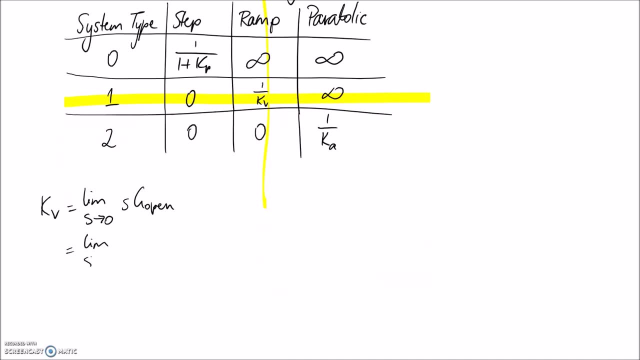 as S goes to 0 of S times, g open. Now we have our open transfer function. It's this one here, So I can go ahead and sub that in, And I missed this S on the front on that one there. So S on the top line. 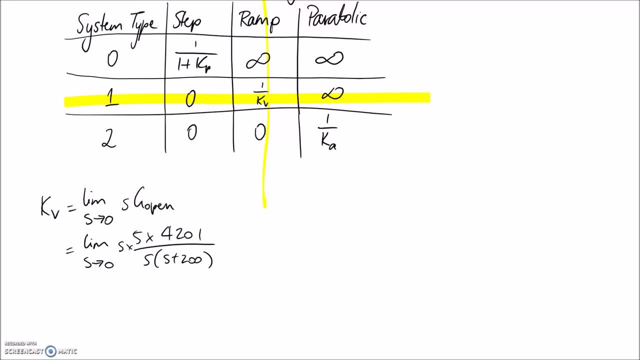 S on the bottom line, they're going to cancel out with each other, And then I'm going to set the limit to 0 for S, so this one goes away And we're left with that. And if you type this into a calculator, you can see that the 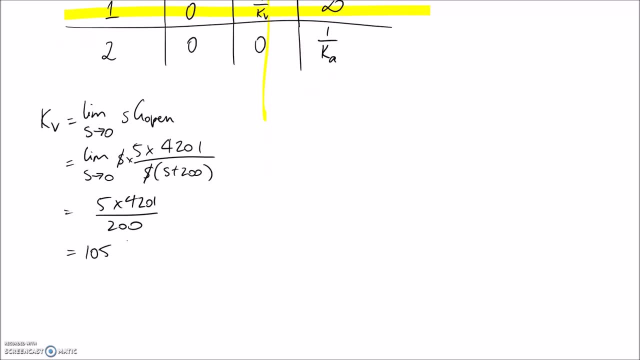 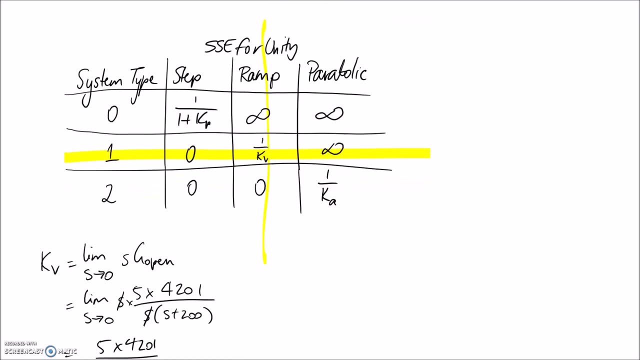 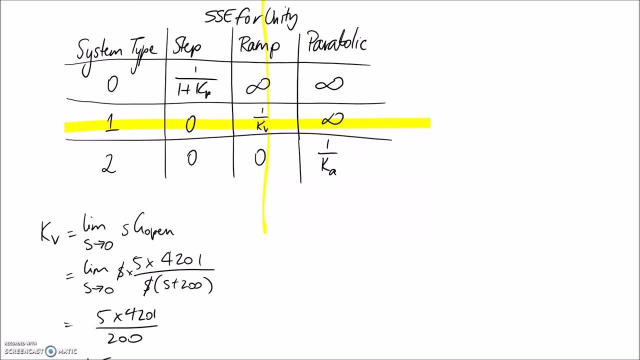 it comes out to about 105 for kv. So this isn't quite the error. This is just the error constant. So what we need to do is this is for a unity ramp input. we just need to do 1 on kv. So I'm going to call this. 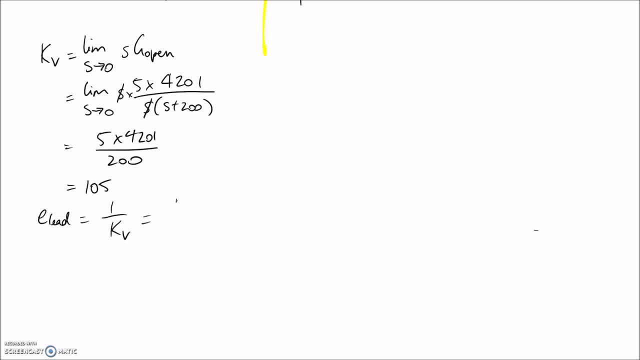 elite at 0.0095.. So remember that what we were aiming for, though I'm going to call this elite lag- It was actually 0.001.. So this is a bit bigger than this value here, So the improvement needs to come. 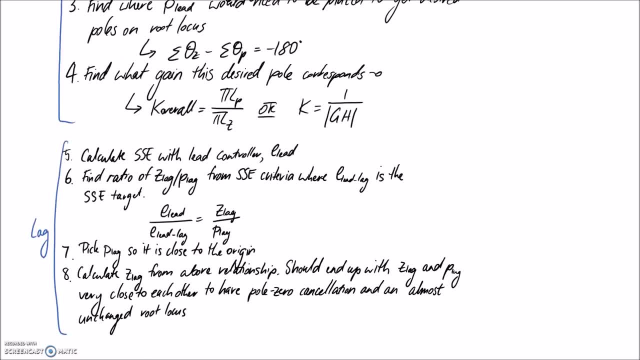 from the lag part of our controller. And if we jump back to our process, what we know is that the ratio of the 0 lag bleh. what we know is that the ratio of the lag 0 to the lag pole is going to be equal to. 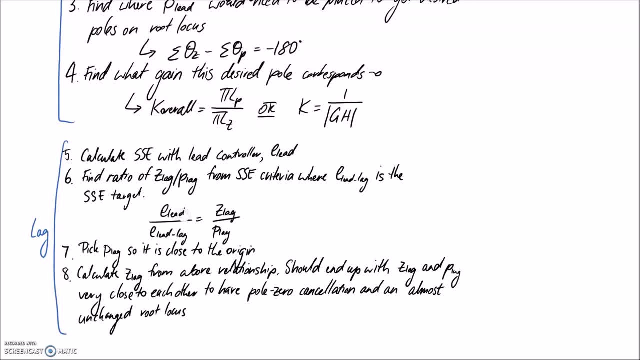 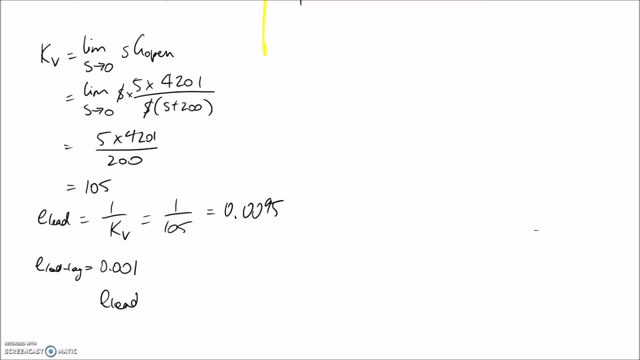 the ratio between the steady state error we have with the lead compared to the steady state error that we have with the lead lag controller. So by applying this equation, we should be able to figure out what the values need to be. So let's pop that in. 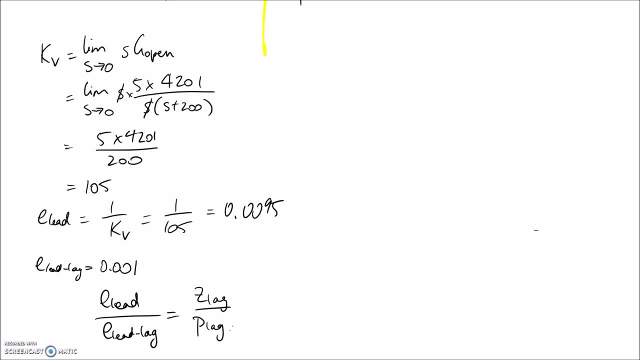 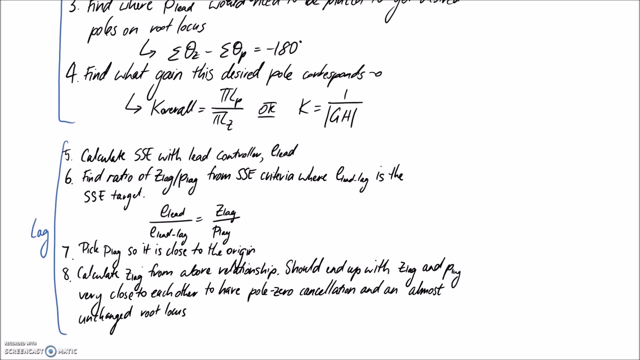 Alright. So we know elite. we know elite lag. These two- here is just the ratio at the moment. So what we're going to find is that we need to pick one of them and then we'll calculate what the other corresponds to. So I'm going to nominate. 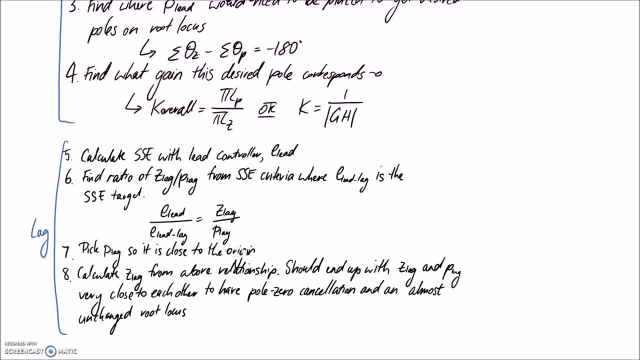 to pick p lag and we're going to pick it to be close to the origin. The reason is these are going to end up being quite small numbers if you pick it close to the origin and that should then end up having pole 0 cancellation between these. 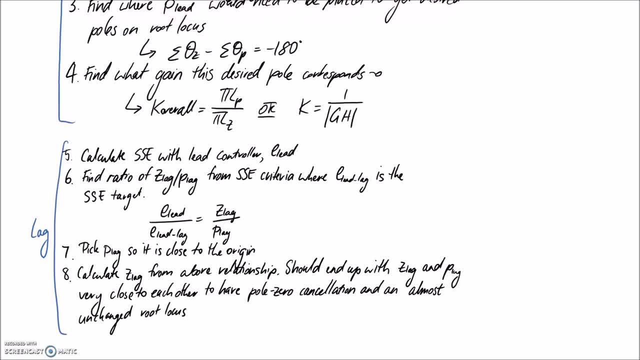 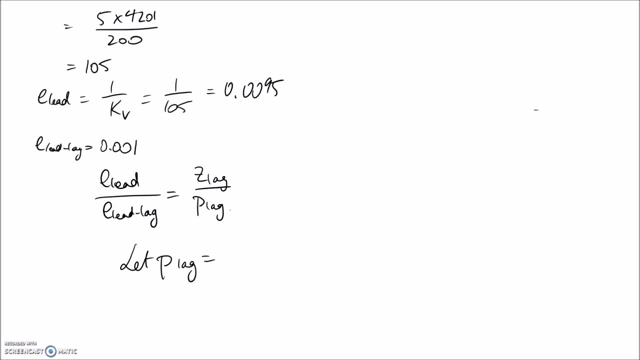 two numbers because they're going to be very small and very close to the origin, So there shouldn't be anything else in there to interfere with them and prevent pole 0 cancellation from happening. So I'm going to pick p lag and I'm going to pick 0.1 for it. 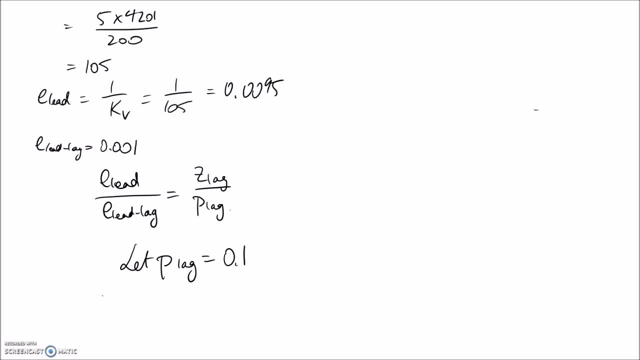 as a small number close to the origin. So if we substitute all of this into our equation, we're going to find that the 0 needs to be at about 0.95 in order to achieve our steady state error requirement. So let's go back. 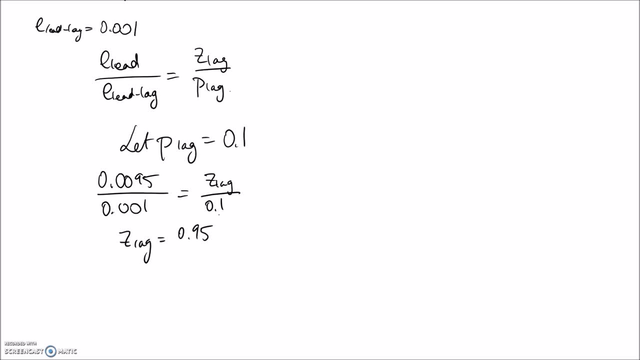 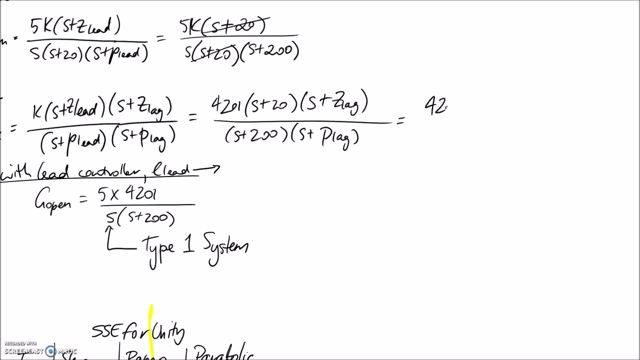 and write the final version of our controller. Alright, filling it up here. So we've now decided on our values. So this one we said needed to be 0.95 and we let p lag be 0.1, and you can see that these are relatively. 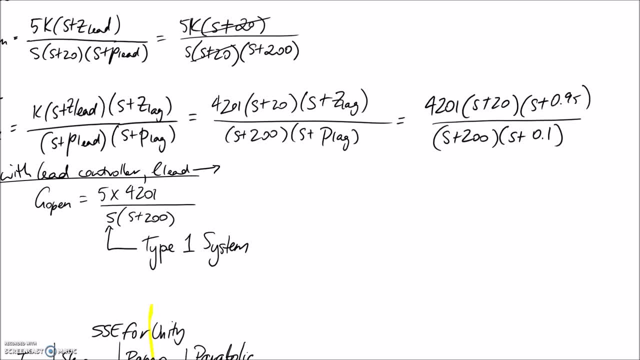 close In a moment. we'll check to see whether pole 0 cancellation actually occurred. But yeah, this is our final value for our controller transfer function of the lead lag variety. So if you're in an exam, that's pretty much where you need to leave it. 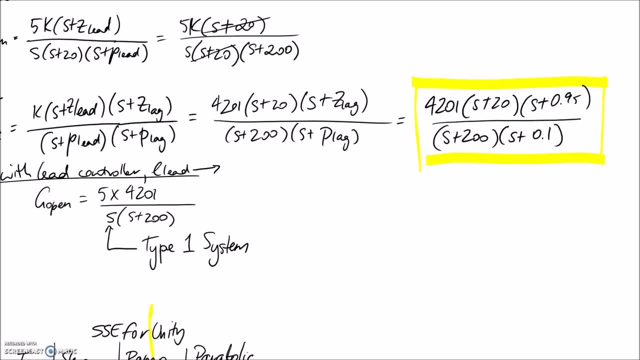 because you don't have any capacity to go and check whether what you designed is actually what's going to happen in real life. But since we have access to that, I'm actually going to have a look. Alright, so let's check our pole. 0 cancellation for. 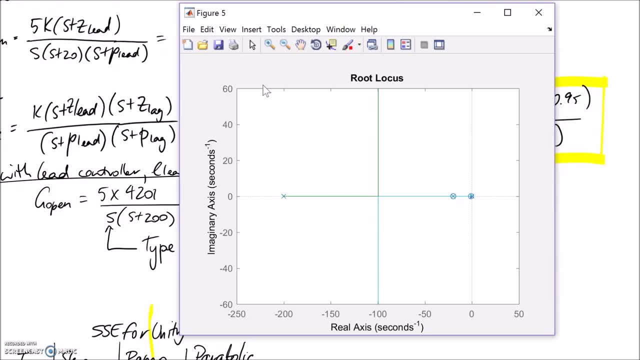 the lag part of our controller. So this is what the root locus diagram looks like and hopefully you can see that it hasn't really changed. We still have our pretty much vertical line here at negative 100 and our pole, we remember, sat on that line. 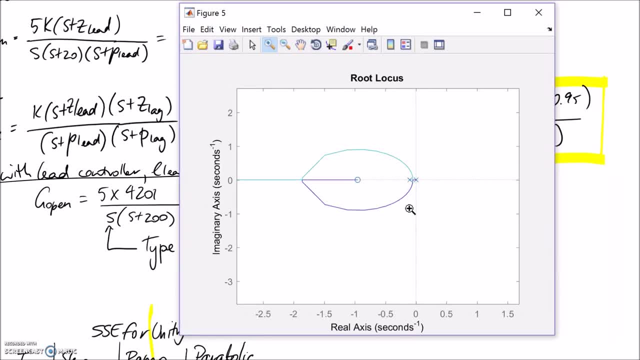 And if we zoom in you can see that we have that original pole, the open loop one at 0, and then we have this pole here that we introduced, this is the lag one and this one here is the lag 0 that we introduced, and they're very close. 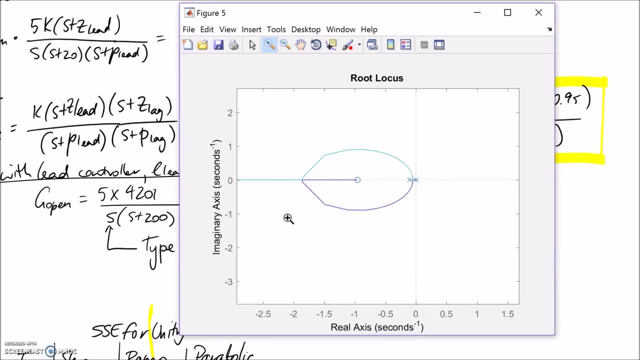 to each other. You can see that there is a little bit of a difference here when we zoom into the plot, but on a wider scale you can't really tell at all that anything changed here. So that's good. that means that we're keeping our transient. 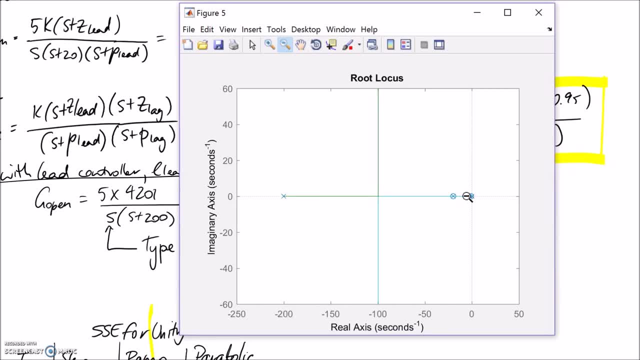 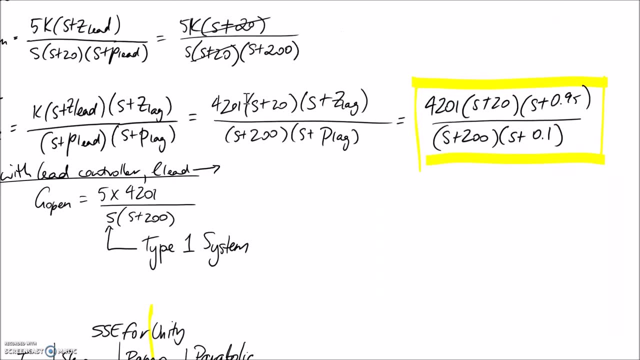 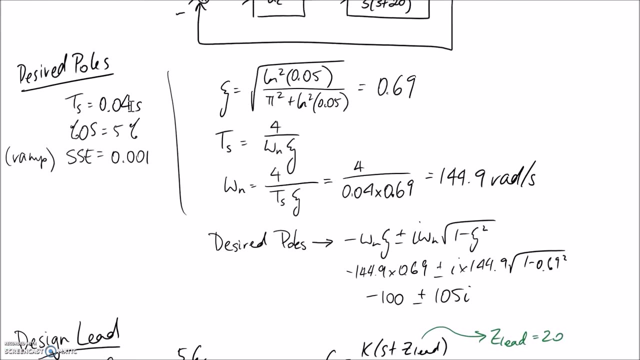 response, which was the settling time and the percent overshoot. So what the other things we were interested in was whether we actually met our criteria, Remembering that all the way back at the beginning, what we were aiming to do was to design something that had a settling time of this. 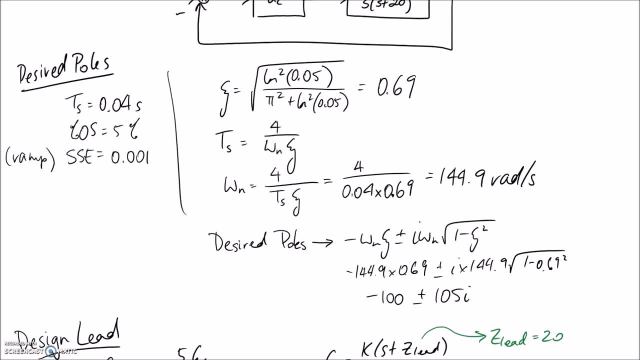 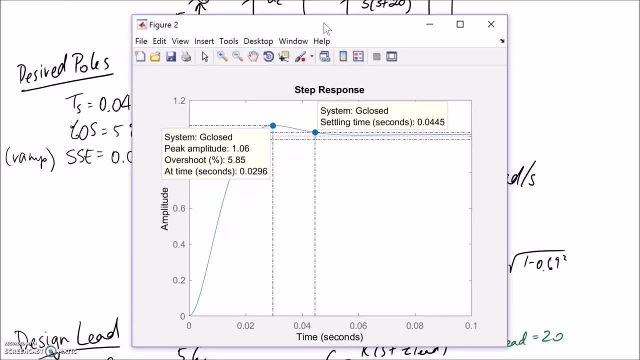 and an overshoot of this for a step input. This part here was relevant to the ramp. So if we just go back and assess the step part to begin with, this is the response that we end up getting. So you can see that the overshoot that we 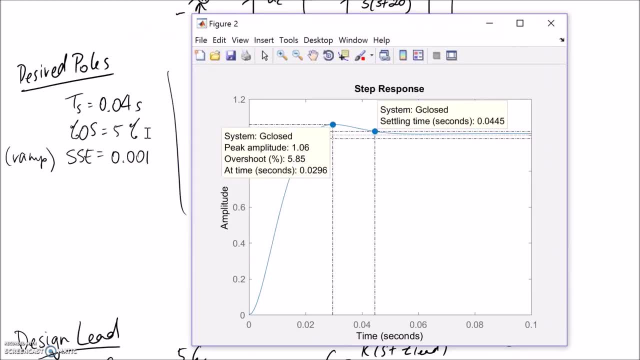 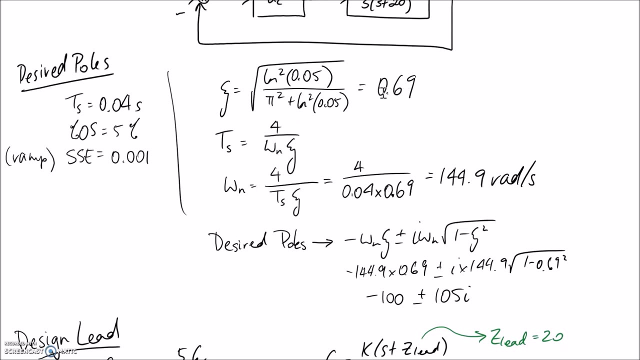 actually got is slightly higher than what we were aiming for, and the reason for this is going to be the presence of the zeros that we didn't account for in our design. So I guess this settling time equation and the overshoot that we have here, they're both. 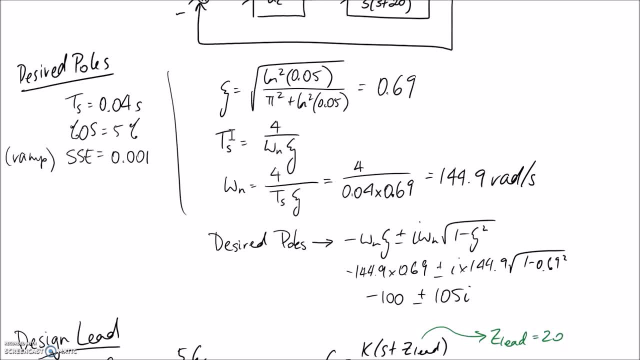 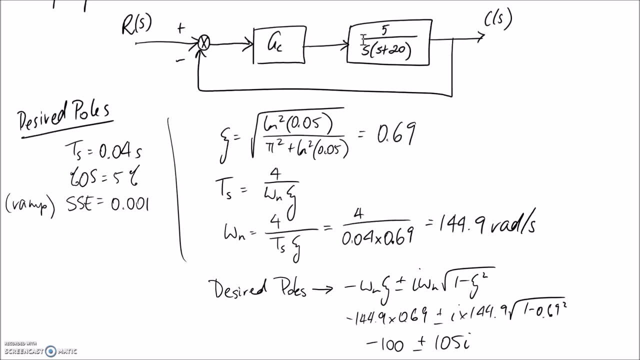 calculated under the assumption that we have no zeros in our system, So that was true at the beginning. we didn't have any zeros at this stage, but as we developed our controller, we did end up introducing them, and that's why we ended up getting a bit.